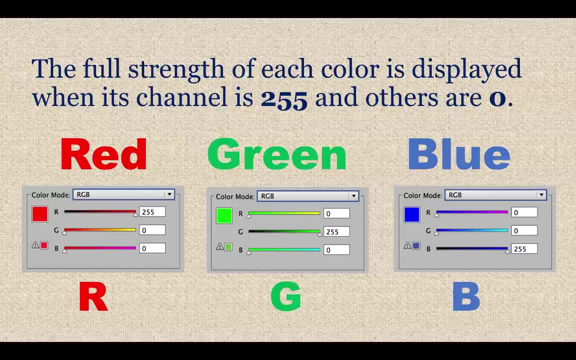 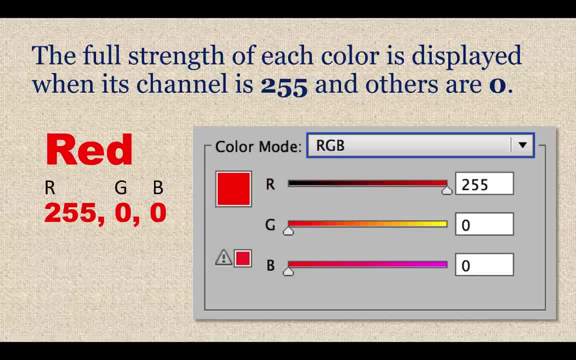 are down, it'll basically show you that true color. So here's an example of the red, green and blue When each channel is up all the way to 255.. Now just to look at them individually: 255, the green and blue are down to zero And we refer to that color as RGB. 25500 in. 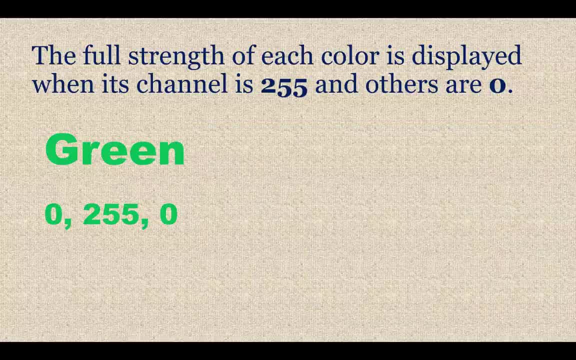 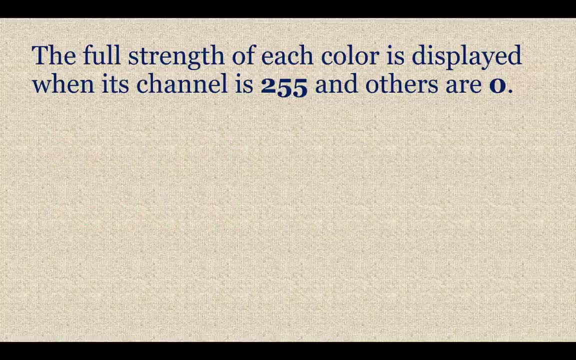 that order And they always go in that order of RGB. Same thing with green. Here's green. Same thing: The green channel is 255.. So when you'd read that it would be 02550.. And then same thing for the blue channel. That's the last channel in our RGB sequence. So when 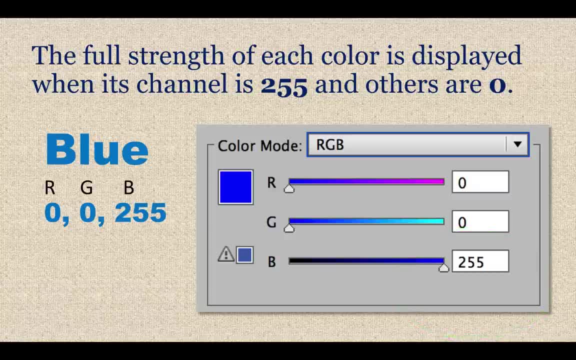 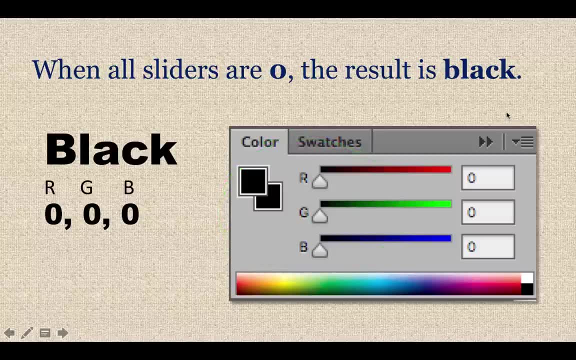 that's up to 255, you'll see the kind of the true RGB blue, which is 00255.. Also, when the colors are down to zero- this is a Photoshop slider here- When the colors are down to zero, you'll see, you'll see black. That means all the, all the lights You could look at. 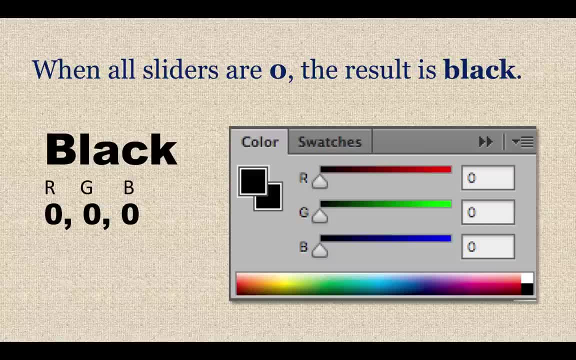 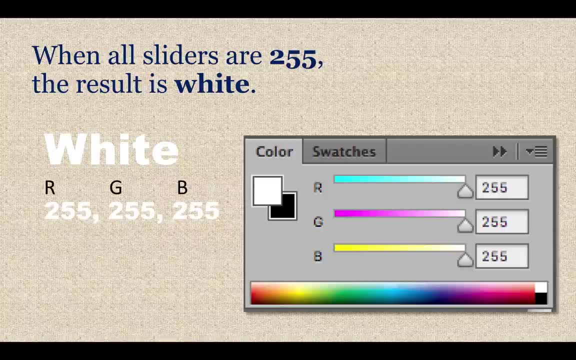 RGB almost as lights. You could say the lights are all off. So when those lights are off, everything's down to black and RGB black would be 000.. Now when it's the other way, it would be light All the, when all the lights are on at the same time. if you picture like a 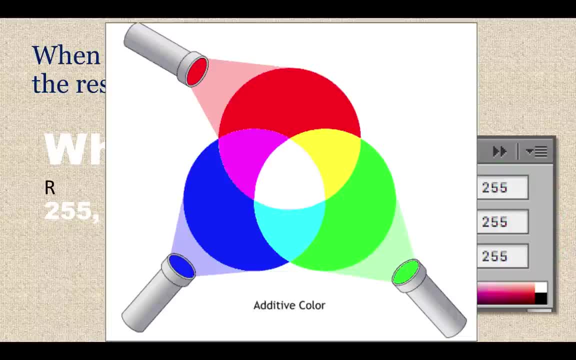 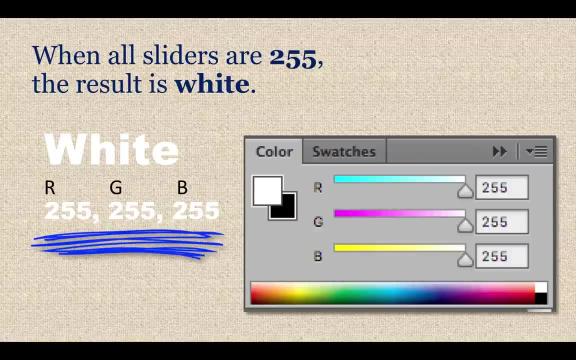 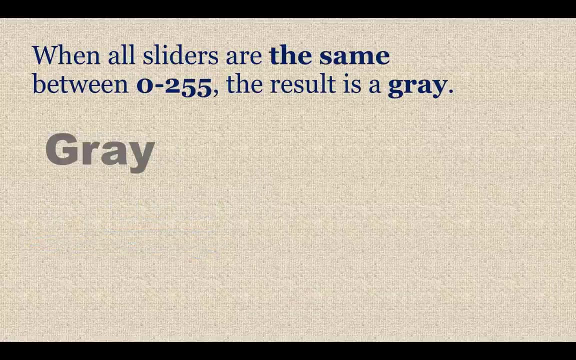 red, green and blue spotlight pointing all in one direction or all at one target. they would basically make one. They would make white when they combine. So that would be 255, 255,, 255 for the RGB equivalent of those colors, And that's their range, Zero to 255 for a total of 256.. And then also just 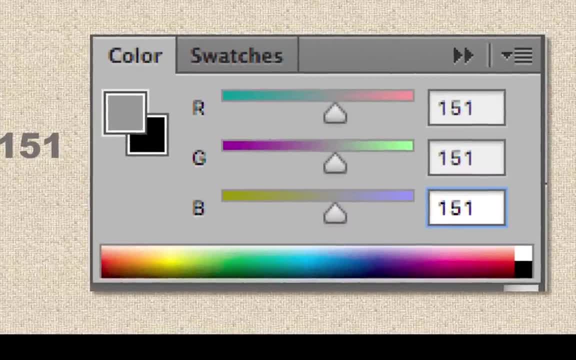 to be aware that anywhere in between a black when they're all off and white when they're all on would kind of make a gray, And when the when the sliders are all at the same point, they'll always make a gray. So higher end on the scale towards the 255, there'll 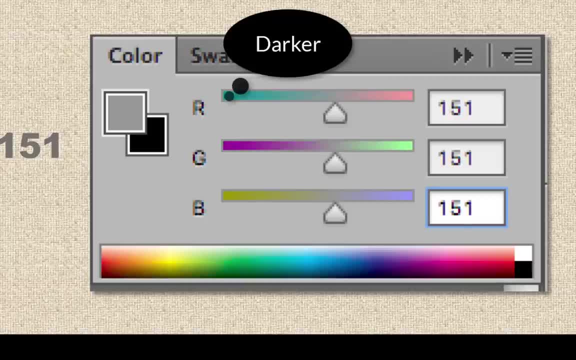 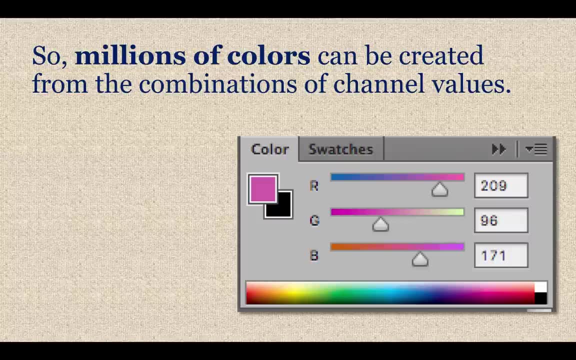 be a lighter gray and down lower on the scale they'll make a darker gray. Now keep in mind also that that these combinations can make millions of color combinations. There's three channels of 255 and basically you could take 255 and cube that and get like 16.7 million. 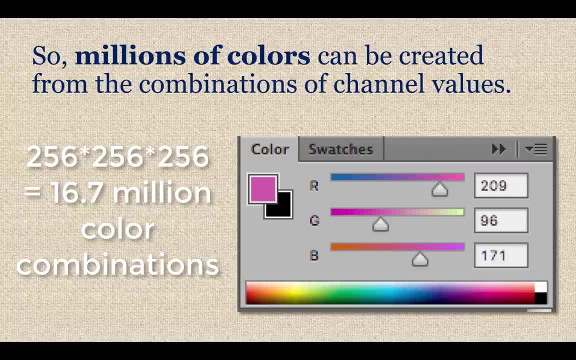 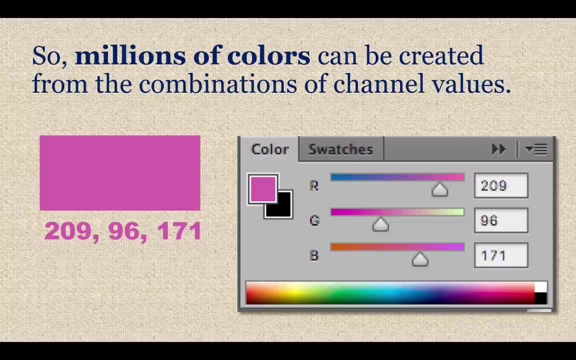 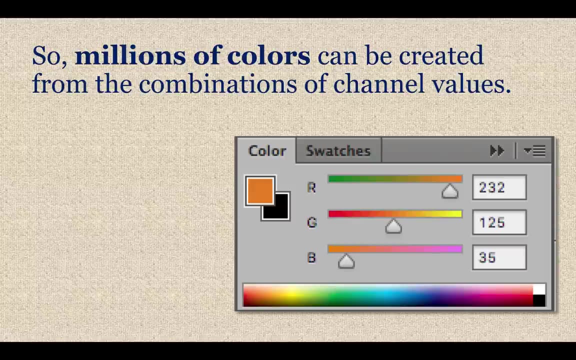 colors that can combine from these channels to create colors on your computer screen. So this is a pink, for example. So that color happens to be 209, 96, 171.. It's kind of a pink color. Here's an orange color which is at 232, 125, 35.. And you can see it, It's 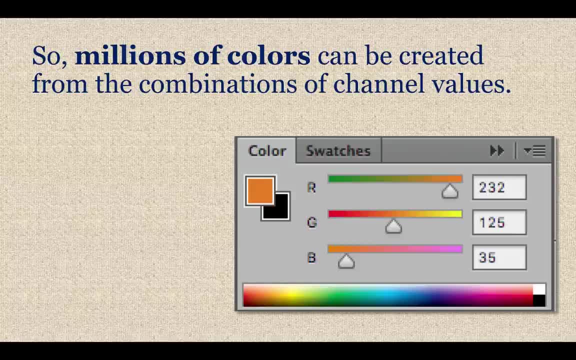 since it's orange, there's a, there's a lot of red in it, There's also green in it. That that kind of makes more of a yellowish color. That's kind of how they have orange, And then there's only a little bit of blue light that's in it, So that makes an orange color. 232,. 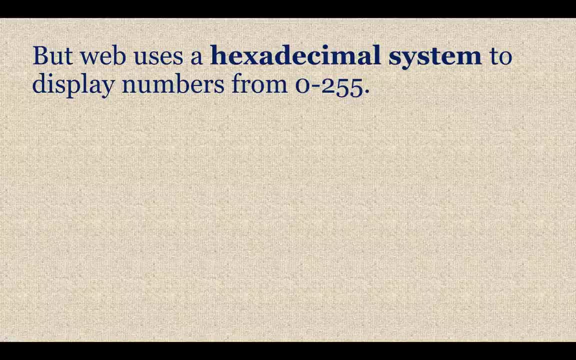 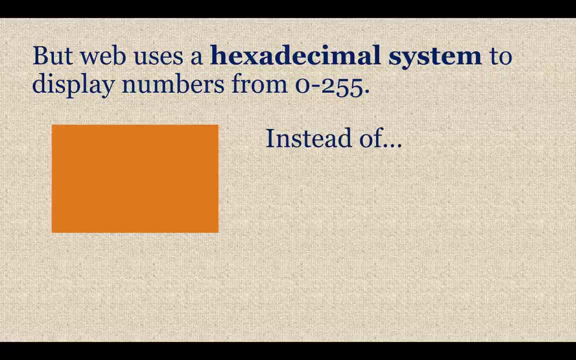 125, 35.. Now, when we work on the web, we use a system called hexadecimal. It's a base 16 number system and it displays the same colors. It's still RGB colors. So here's an RGB color of 232, 125, 35.. The one we just looked at 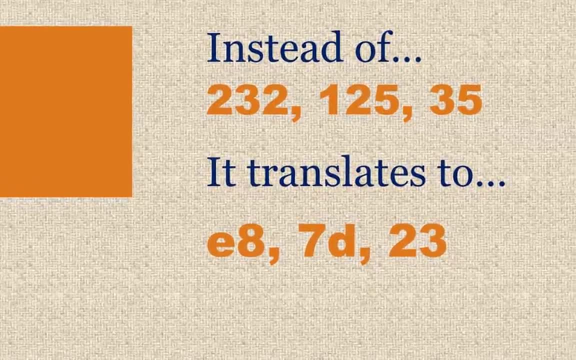 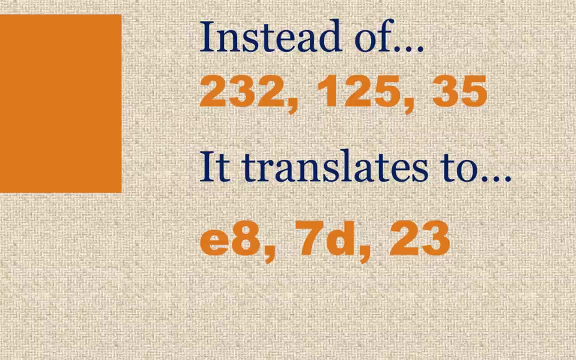 Now in hex it's E87023.. The only difference is that it uses different letters and numbers and there's only two digits for each color instead of three. Whereas in RGB there could be three digits for each color, In hex there's only two, and there were will only be two. 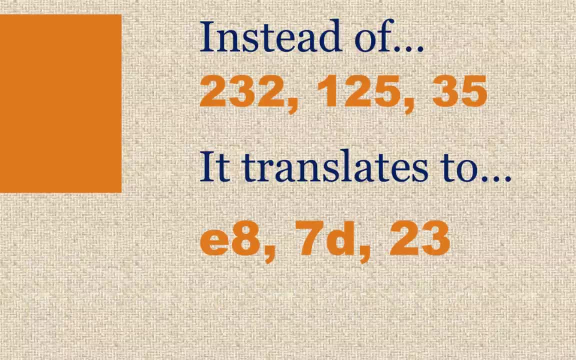 It won't go higher than that. Um, it doesn't necessarily make things easier to translate, but I just want you to understand how hex works a little bit so you can understand that it's really just RGB color. It's just a different way of describing it. It's kind of like taking 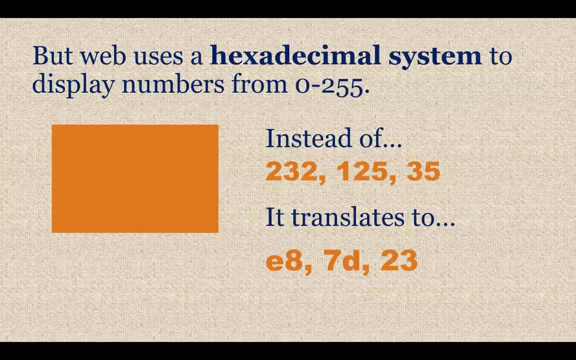 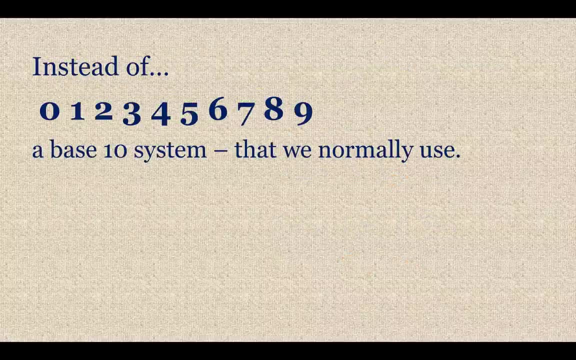 the you know state names like New Jersey and Pennsylvania and abbreviating them to you know NJ and PA. They mean the same thing, It's just you'll see them. you'll see them in a different way. Normally we have a base 10 number system. That's what you're familiar. 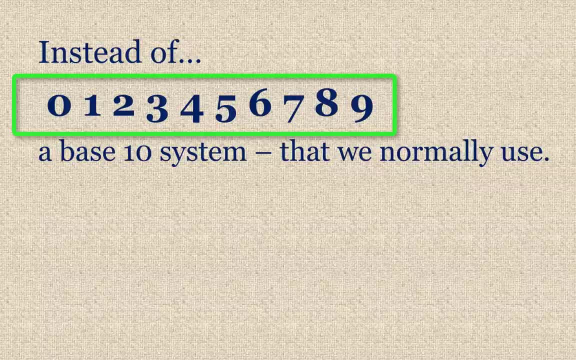 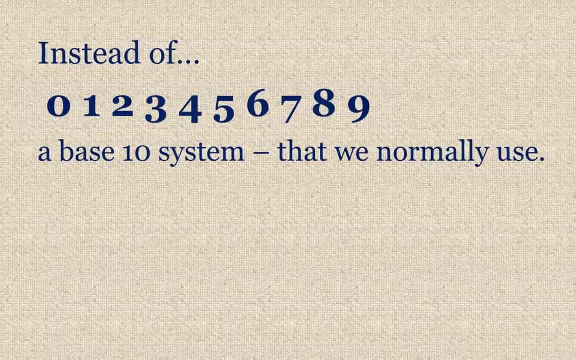 with. We have digits zero through nine, and all our numbers in our system are composed of those integers, zero through nine. So any number we have is only going to have those numbers, those 10 numbers with zero included. Now in the base 16 system there's 16 numbers. 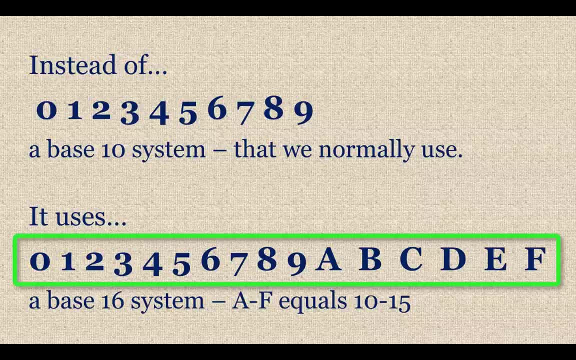 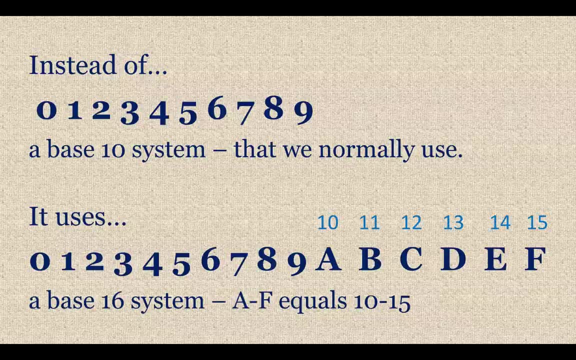 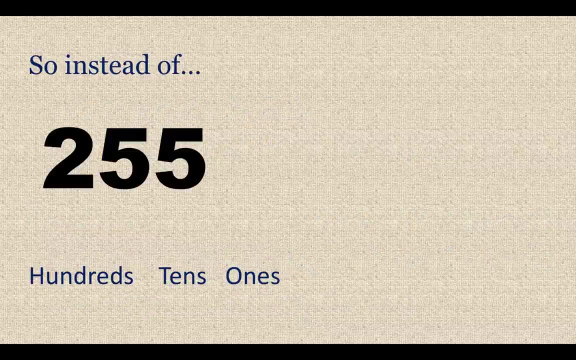 including zero When they get to 10, they want to keep them to be single digits, and there's no single digits after nine, so they use letters. So they use A, B, C, D, E and F, and they basically translate to 10,, 11,, 12,, 13,, 14 and 15, and that's as high as it goes. So, instead of 255,, 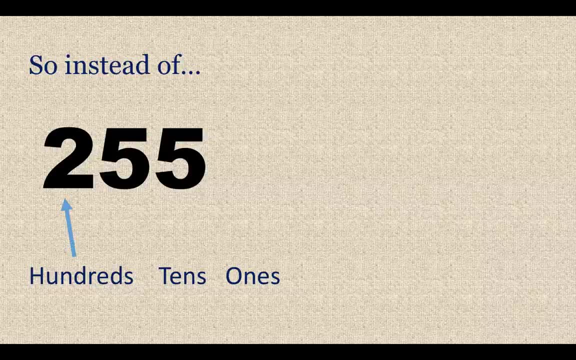 let's say an RGB channel is 255, you know we would normally read that number in hundreds. You know there's 200, there's five tens and there's five ones. That's how we get 255.. That's our base 10 number system. 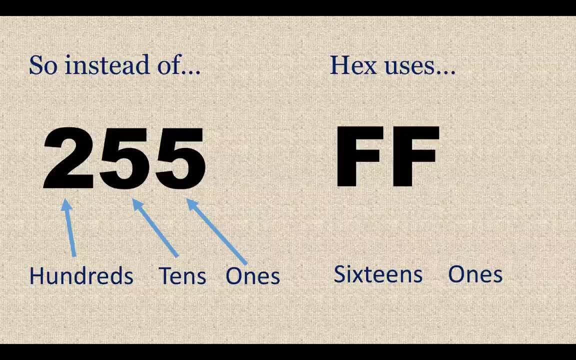 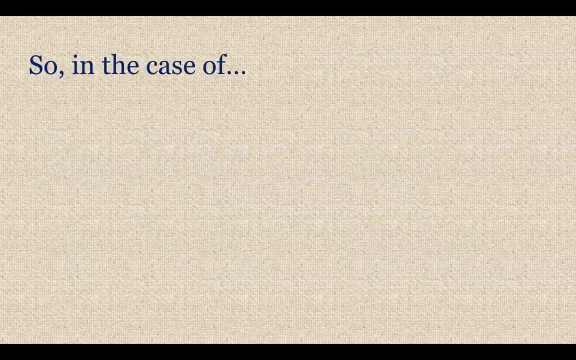 The decimal system. they basically use a system where there's a 16s place and a ones place. So there's, the first one is 16s, the second one is ones, and that actually translates, because F is equivalent to 15.. So there's 15 16s and there's 15 ones, and that's how we get 255. 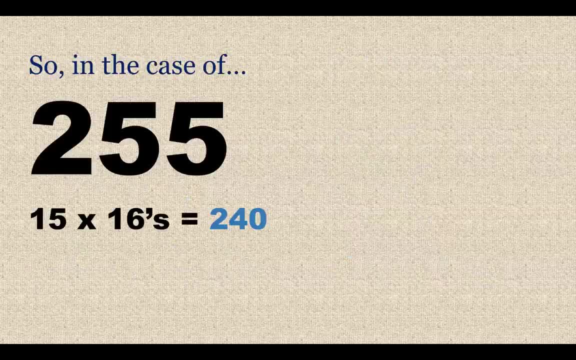 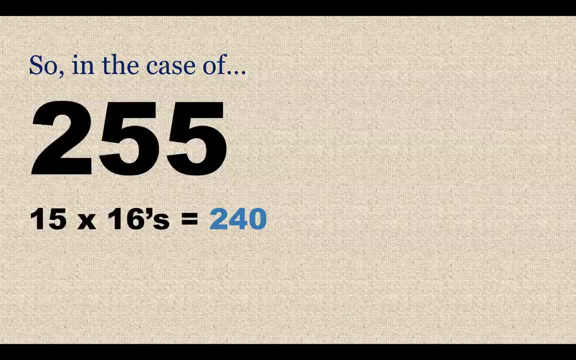 So here I'll kind of go through it. There's 15 16s which, if you do 15 times 16, it'll come out to 240.. Now you can't do any more than that, since the number system only goes. 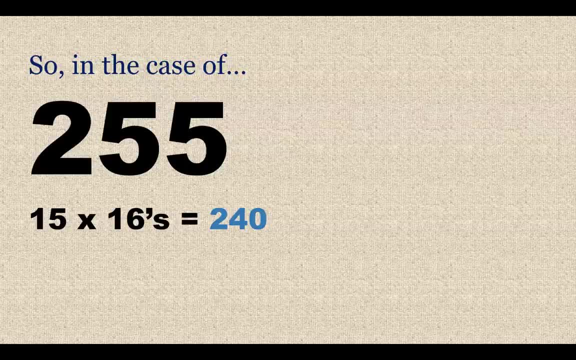 up to 15.. So, as far as, as far as digits, you can't have more than that anyway. So that's the highest it'll go. So there's 15, 16s, and then after that you could only have the highest. 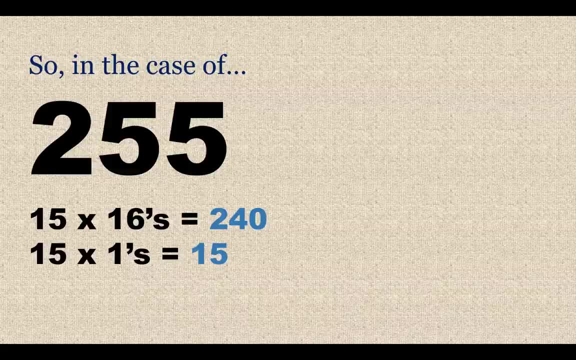 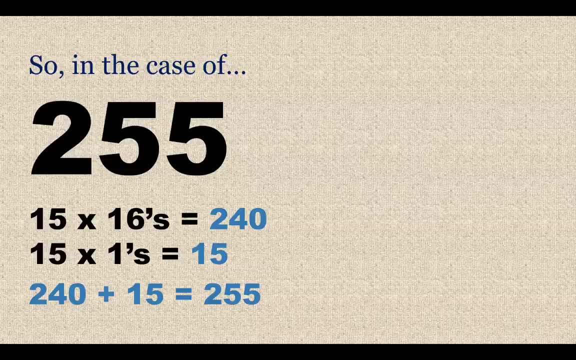 number, 15 ones, and that makes the highest number in the RGB scale. So you get 240 plus 15 and that comes out to 255.. So there's the 16s place and there's the ones place. There's the 15 equals F. 15 equals F. That's how we get this color to basically be FF, and it's. 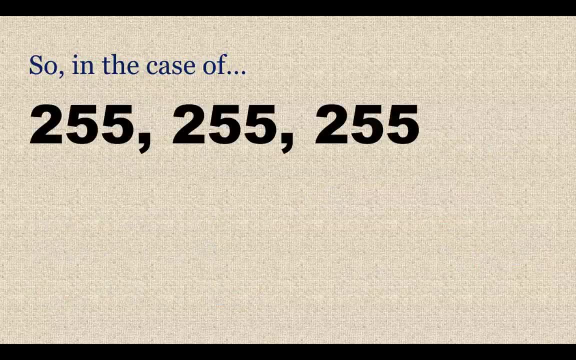 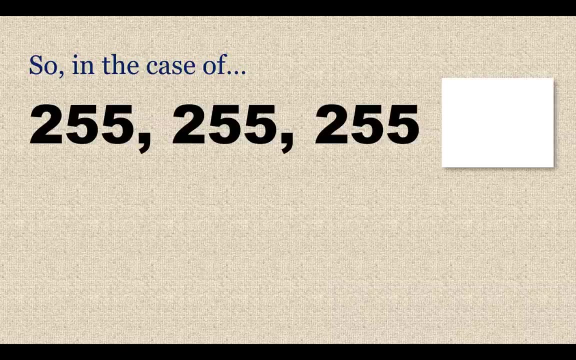 not a color, It's really. one of the channels is FF. Color itself would be 255, 255, 255, because we have three channels, So this would actually be white. Now in hex it would show up as FF, FF, FF. Each pair of letters is equivalent. 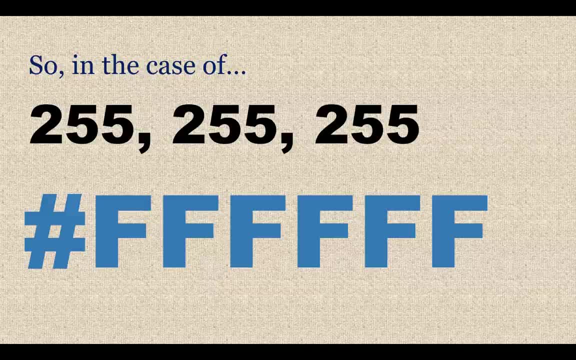 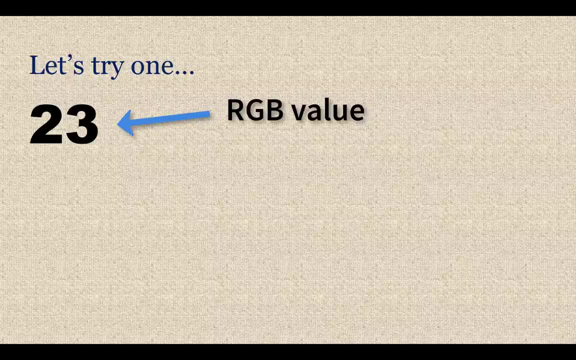 to 255 and we put a pound sign in front of it to indicate that it's a hexadecimal color. Now let's just try one, just to just to see if you could figure it out. So if we had an RGB channel that was 23, now that would be pretty low. That would be a darker color. 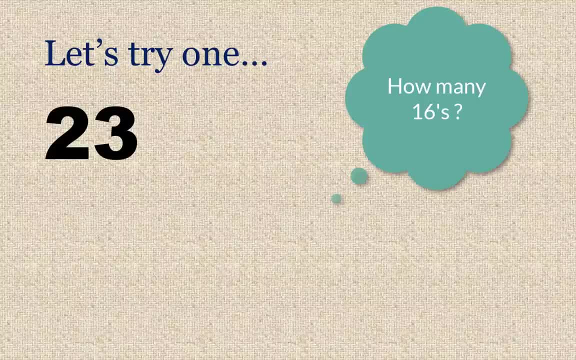 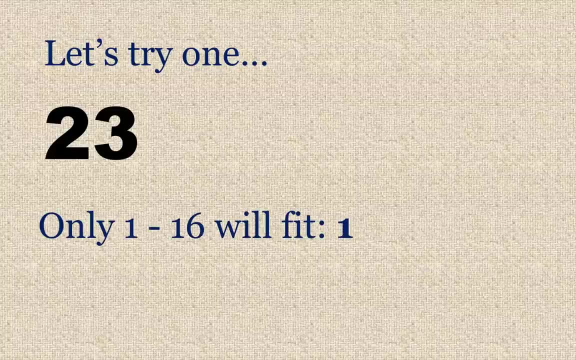 And obviously if you know a little bit about math, you know only one 16 could go in there, because two 16s would be 32.. It would be over. So one 16 will fit in there and then whatever's left over- 23 minus 16,- there would be seven ones left over. That would basically be your. 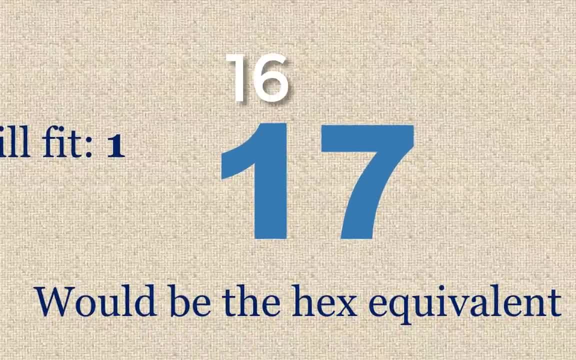 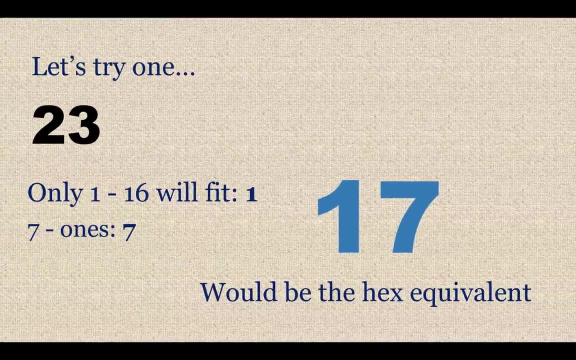 hex number. Your hex number would be 17.. There's one 16, and then there's seven ones, and that comes out to 23 in terms of a number, but you'll it'll be translated as 17 in hex. Here's another one. Here's a larger one, which would be down towards the other end of the. 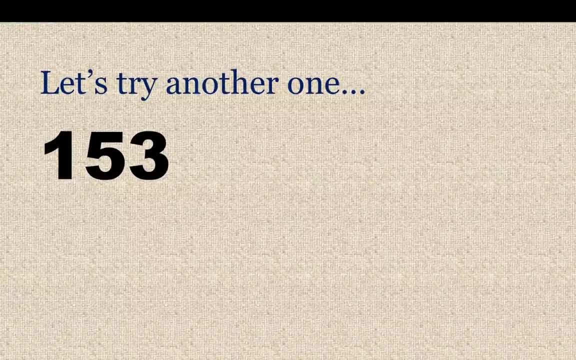 scale or a little more past the middle, 153.. Now, if we try to fit 16s in here now, you might say, well, I don't know how many 16s would go in there. Well, you could start with. 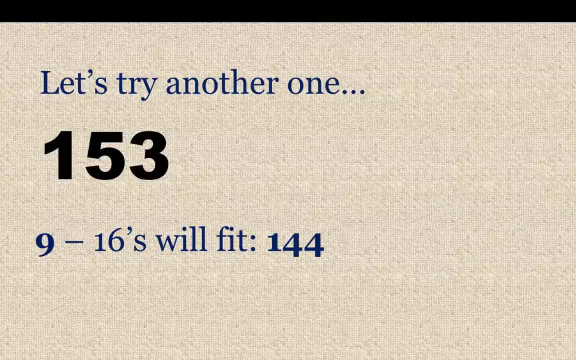 10.. You could say 10 times 16,, that's 160.. Does that fit in there? No, Well, let's go down one. Can nine fit in there? 144.. Yes, it can. So we know that the first digit would. 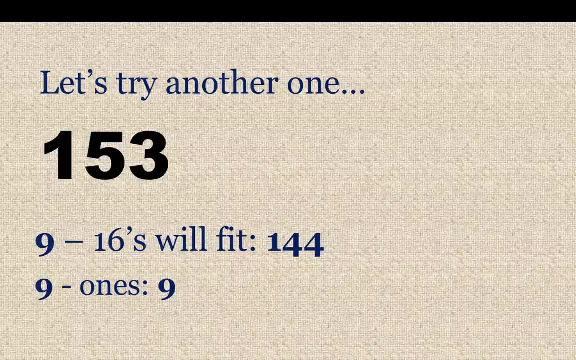 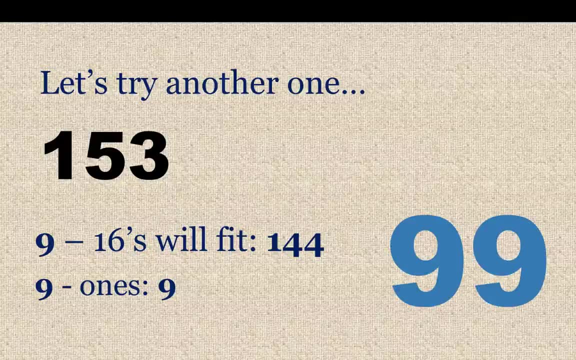 be nine 16s, and then we could just subtract the difference. The difference would be nine, because it would take nine ones to get up to 153.. So that number would basically be 99.. Nine 16s, which is 144, and then nine ones, which will take it up to 153.. So that's the 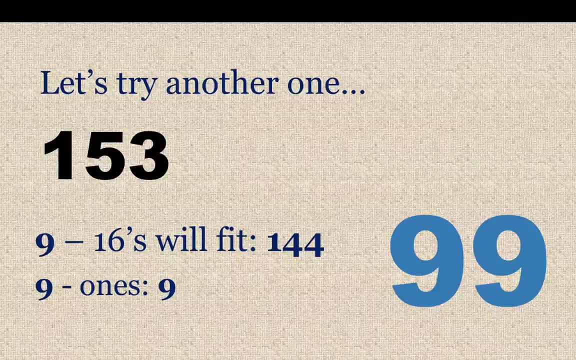 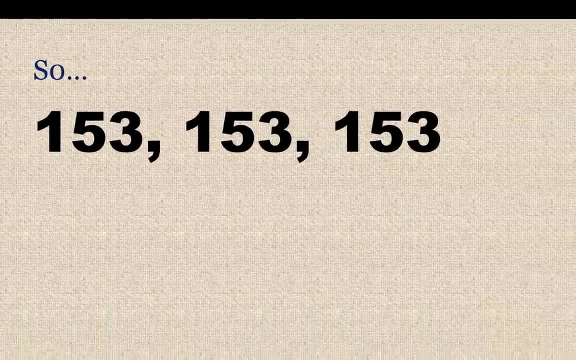 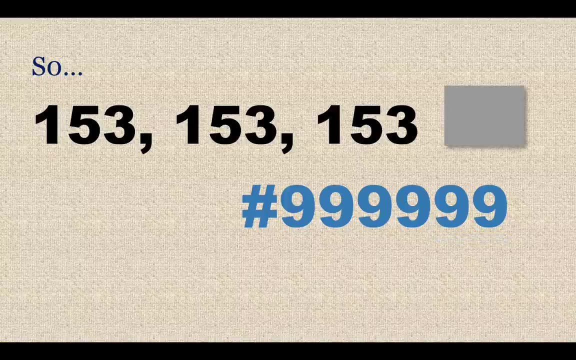 equivalent of the RGB 153 color is 99 in hex, So 153, 153,, 153.. If you're looking at the whole color, not just one channel, that would be 999999. with the pound sign in front of it, We would see that that would be a gray color. Now we can abbreviate this whenever. 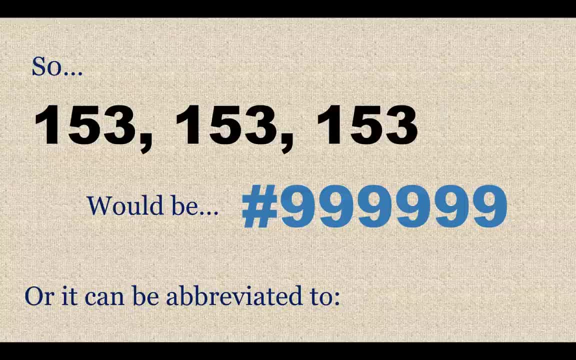 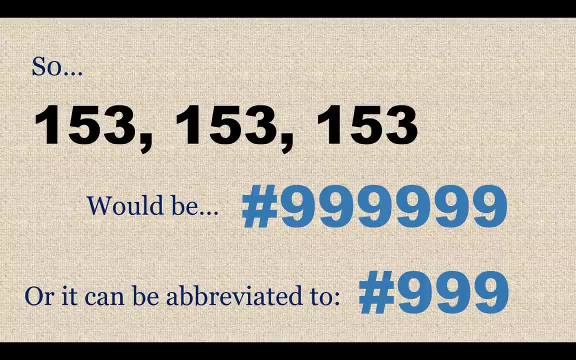 we have the same pairs Of colors that are the same, like 9999, we can actually abbreviate it and just use the first one. So whenever the second, uh, the second digit of these two digits are the same, you can, you can abbreviate it, You can put it 999 to kind of shorten that, So you don't. 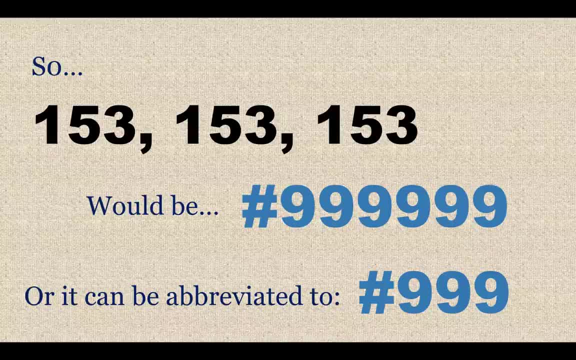 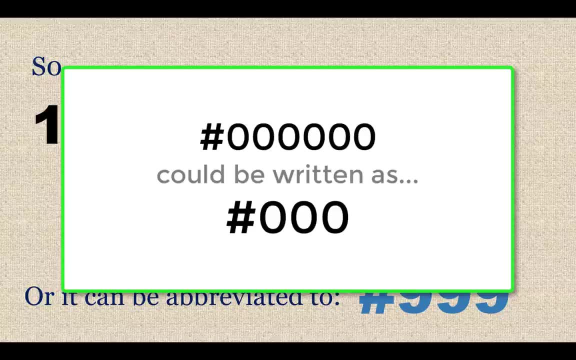 have to do 9999,, just like if you had 000000, you would just put 000.. It'd be kind of almost like using first names, in a way, And we'll see that when we uh, when we use that in. 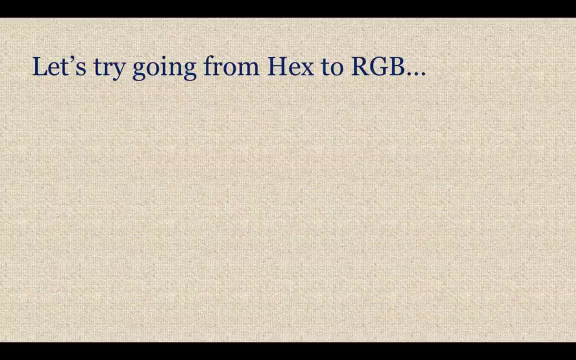 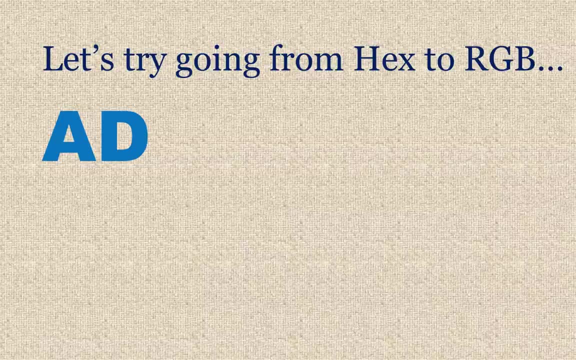 CSS. So we're going to abbreviate that a little bit. Um, let's just try the other direction, going from hex to RGB. So here's a hex number. You might look at that and say what the heck is AD? Well, if you just know that, that the first digit is the sixteens, you can know. 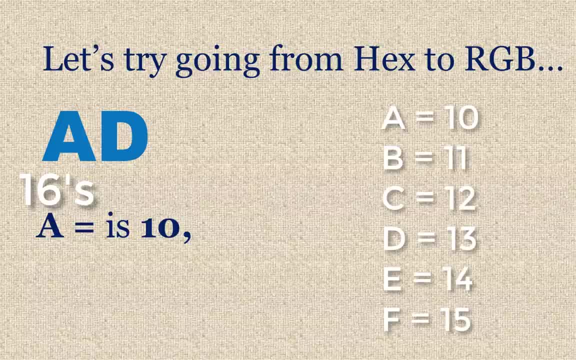 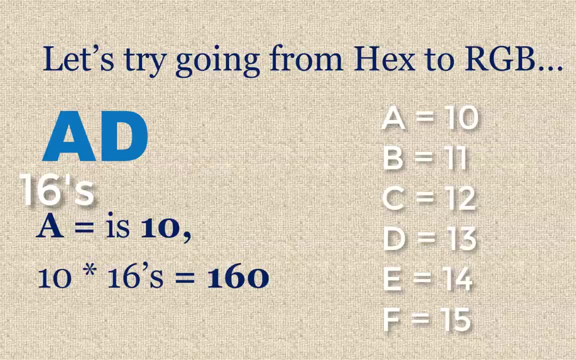 that a is 10 because in our number scheme it basically goes up to nine And then after that is a, which is 10.. So if we know that there's 10 sixteens, that means that there's one. the first number would be 160 and then the ones would basically be 13, because D happens. 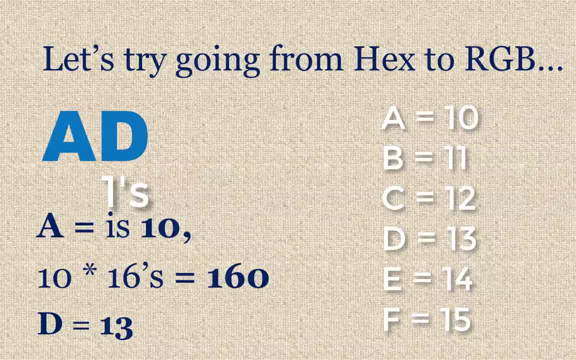 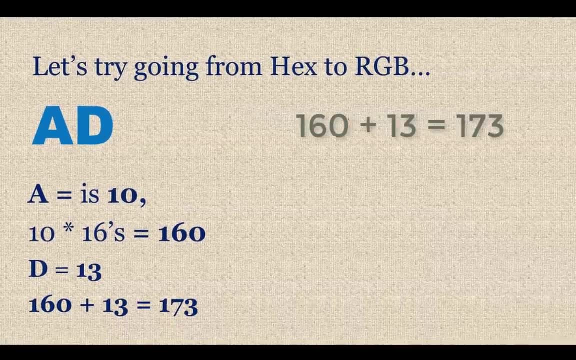 to be 13.. A, B, C, D, that goes up to 13.. So there's 13 ones and there's 10, sixteens, which is 160.. So that color would be 173.. That would be the equivalent of the RGB 173.. Now, if I went, 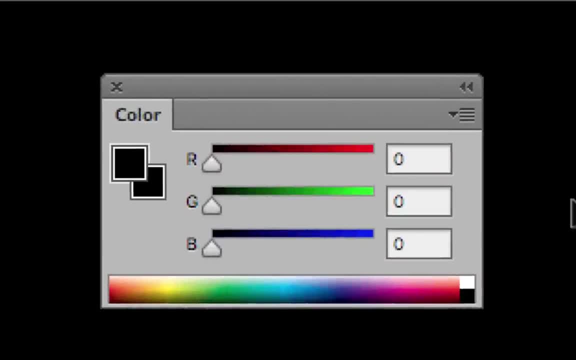 into Photoshop just to take a look at this color slider. you know, if I wanted to check that out, I could go here and put in 173, because it was our first one. I'll put in 173 and I'll leave the others at zero, And you could see it. it kind of makes a dark red And if 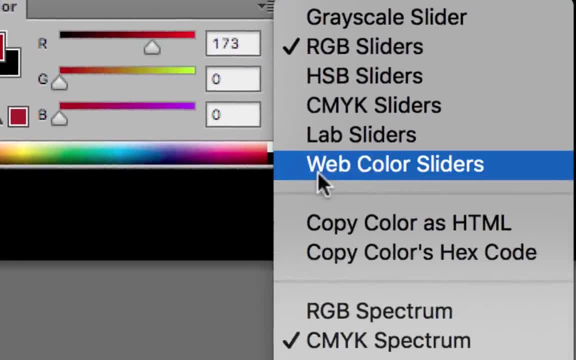 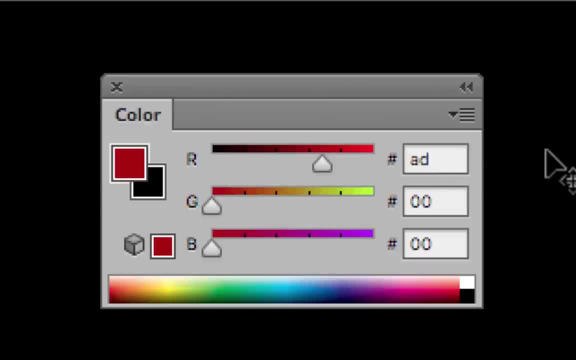 I wanted to see the equivalent in Photoshop. I could go here and go to one, So web color sliders- and I could see that it is a D, so it does the conversion there. So if you have any software that has sliders, I mean even word and PowerPoint have sliders. 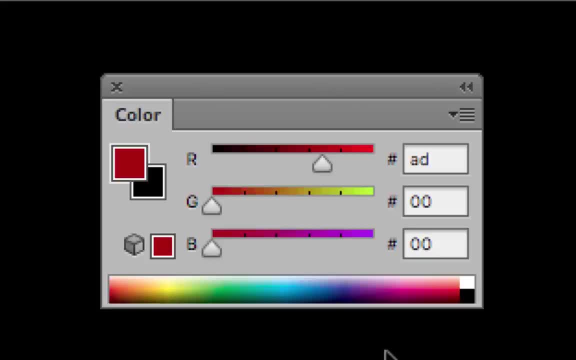 you can figure out what they are When you look at this. if you kind of zoom in there, you could see that they have little ticks there. There's actually six spaces and that kind of indicates web safe colors in the early days of the web. Um, since everybody was looking, 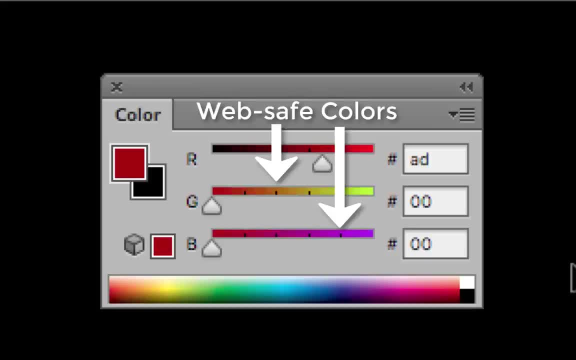 at websites on sometimes older monitors, old PC monitors and things like that, that couldn't display a million colors. They used to recommend doing logos and type in web safe colors. and web safe colors meant that they were colors that could display on any monitor, even if they only displayed thousands. 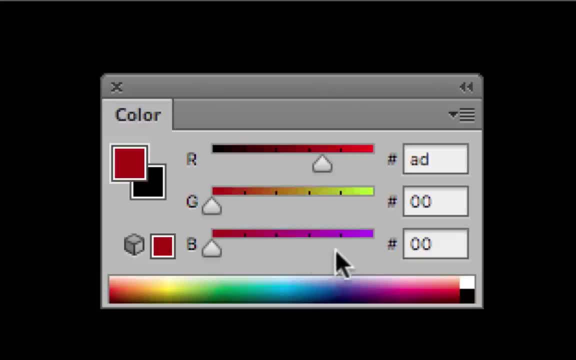 of colors. So what they used to do is take the, these websites, these RGB colors and break them down into six spots. So there was basically six spots on here. that would make maybe about two, 16,. uh, there would be six, six, six And if you put them, if you cube, 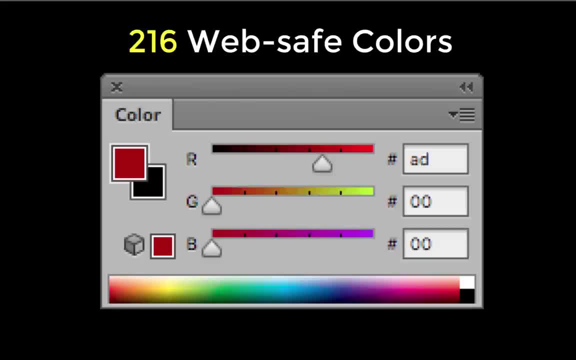 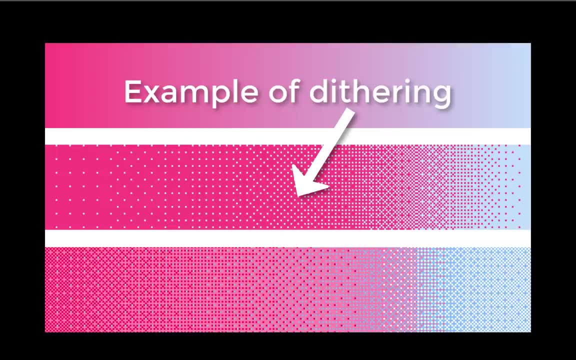 that it would come out to two 16. So you'd basically have 216 color combinations that you that were considered web safe. that wouldn't dither. What would happen is they would dither. They'd get little spots on them if they would, uh, if they would show up on a monitor that couldn't 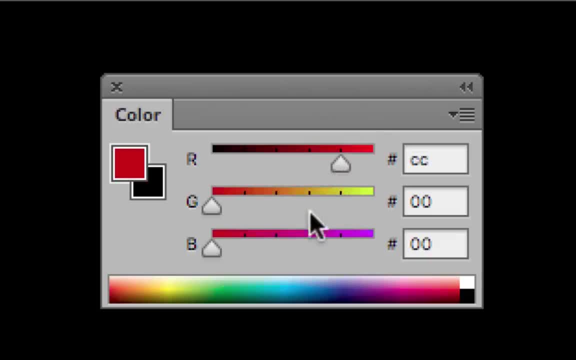 display the colors. But if you keep these sliders on those little ticks- and even in Photoshop they still kind of have these on here- So what you'll see is you'll see numbers starting from the bottom, from zero, zero, zero, three, three. The next one would be six, six. 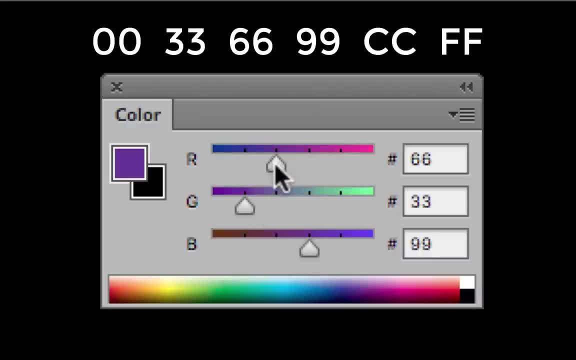 The next one would be nine, nine, And then the next one would be CC and the next one would be FF. So you would only see those numbers, those six numbers, in various combinations to be web safe. So if you ever saw colors that were that were only with zero, zero, FF, three. 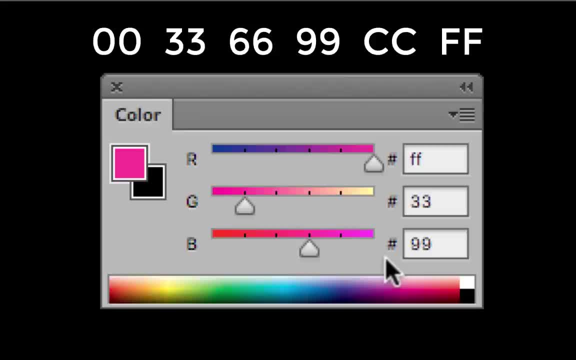 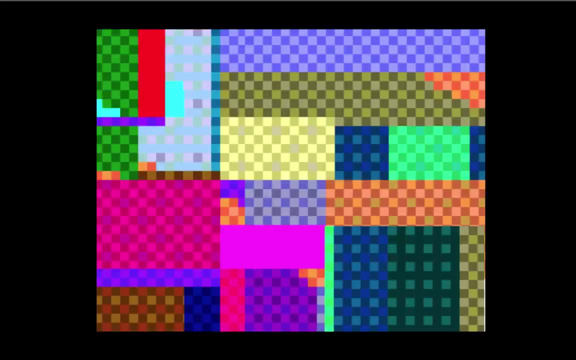 three, six, six, nine, nine and CC. they were web safe colors and they were recommended to use with logos and type that they wouldn't dither. They wouldn't get little splotchiness um in them when, when you would see solid colors. So just be aware of that. Now we don't. 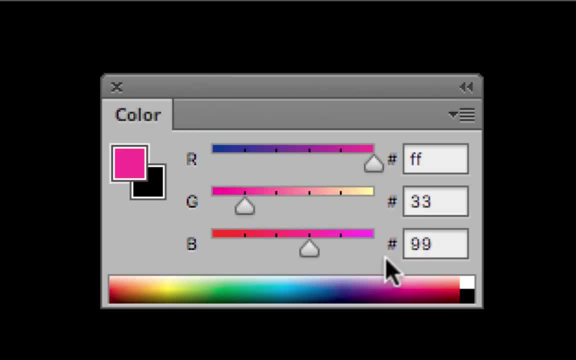 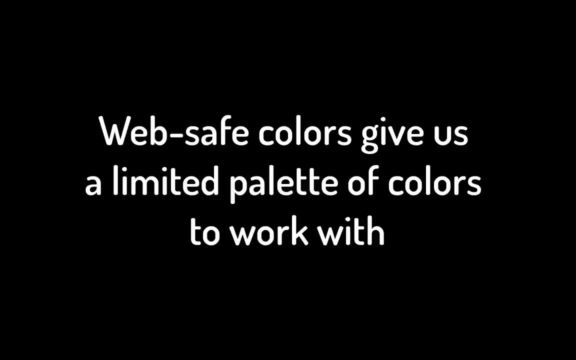 have to use web safe colors anymore because we don't use that monitors that only display thousands of colors. But But the one reason we would use web safe colors is it gives us a limited palette to work with. So you know, 16.7 million colors is a lot to choose from, but you might have us, you. 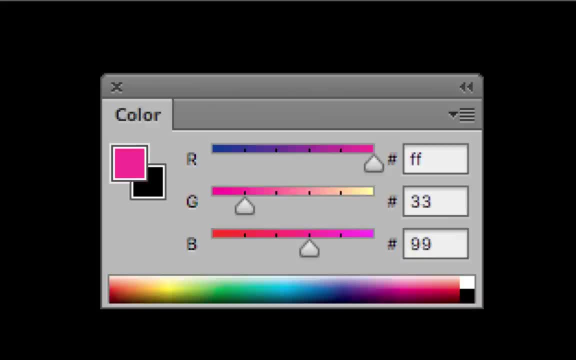 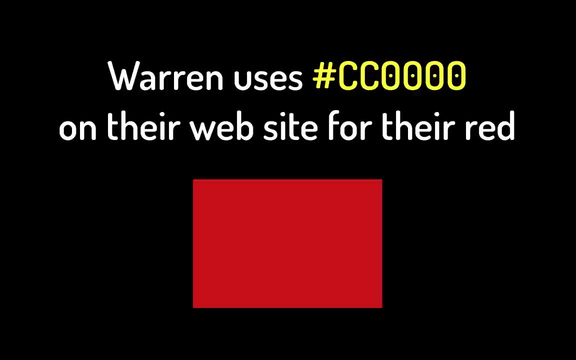 know kind of like the way we use PMS colors in print. We have specific shades of colors that we might use for something. We might have a specific PM or a specific web safe color that we might use for our headlines, for our type, for background colors and so. 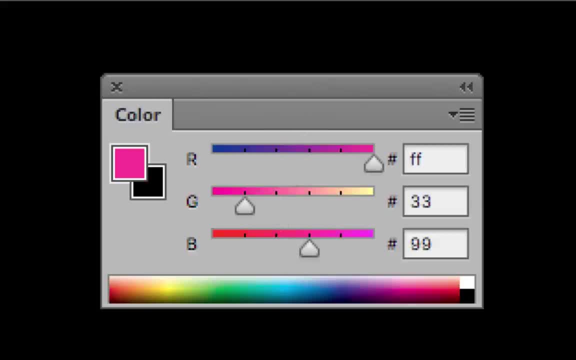 on. So you still may use web safe color color- and you'll still see that in programs like dreamweaver and flap, And even brackets may show you web safe colors when you go to click on there and use a slider. So that's what web safe color is. You don't have to use it, but it's kind of helpful to. 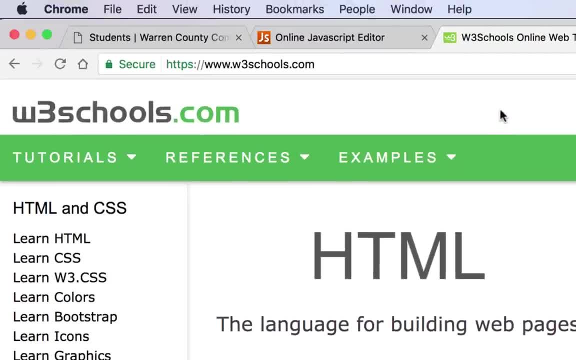 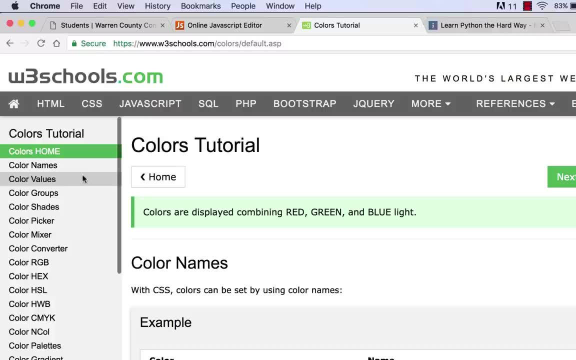 use it. I'm going to go into w three schools and if you want to learn a little bit more about color, they have a section right on their homepage called learn colors and it has all kinds of areas here to go into. but they do have hacks here. They talk about RGB. 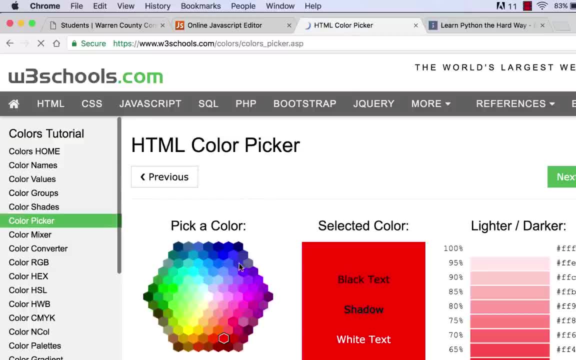 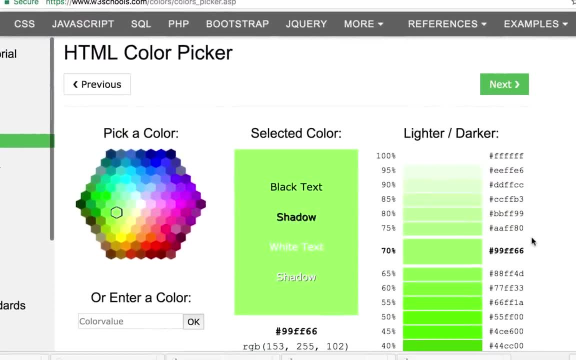 and they have some tools like a color picker, where you could kind of, you know, click in and find colors if you ever need to. You know, if you didn't know what the color was, and it'll tell you all the. you know the hex, these are all hex colors over here. Um, you're. 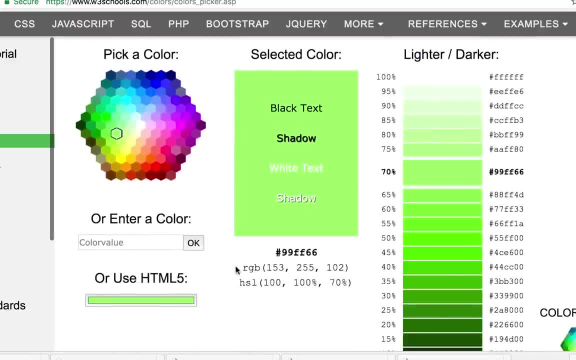 seeing percentages. These are the RGB equivalents. Keep in mind in web, when we we can use RGB in web now and we could even use it where we have something called alpha RGB a will, where we can also make it adjust the transparency. So you'll see that and we'll talk about that.